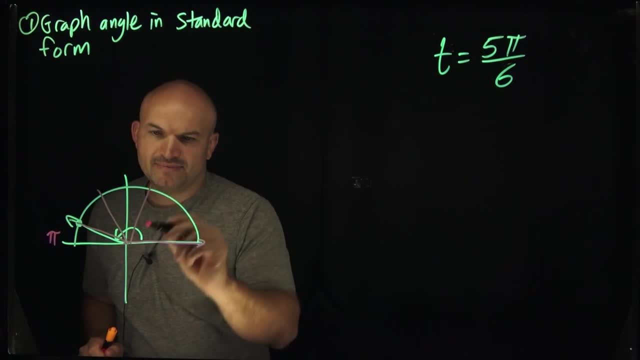 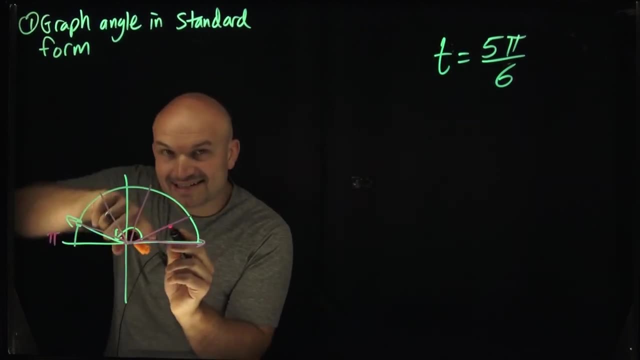 up into six equal sections. I'm not going to be the best here, but hopefully you can see that one, two, three, four, five, six, right. So I'm going to go five of them, right. So you can see. that's why I kind of did this arrow where I'm going to rotate and then 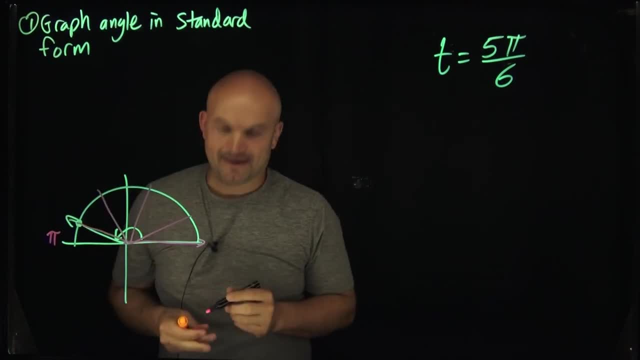 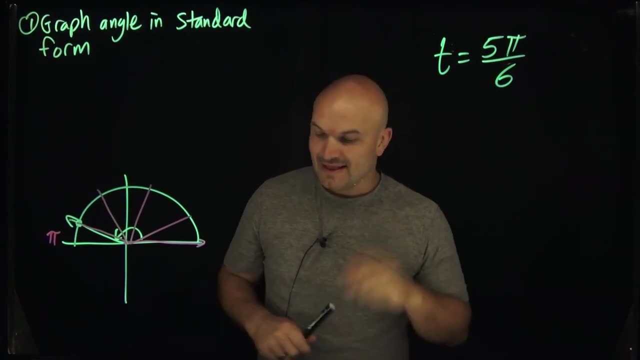 rotate it one, two, three, four, five. That's where it's going to lie, all right, Okay, so that's the first step, And a lot of times you can do this in your head, which is the good thing. It just takes a little bit of practice to do this. The next step that I 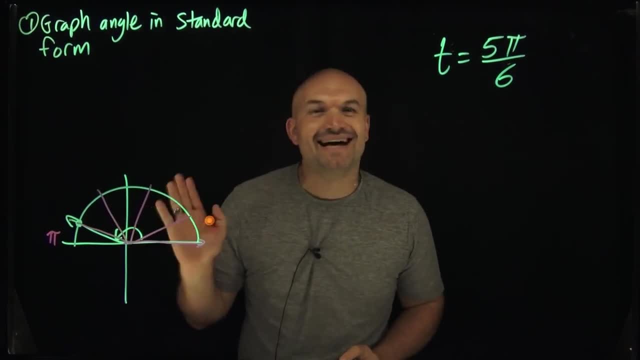 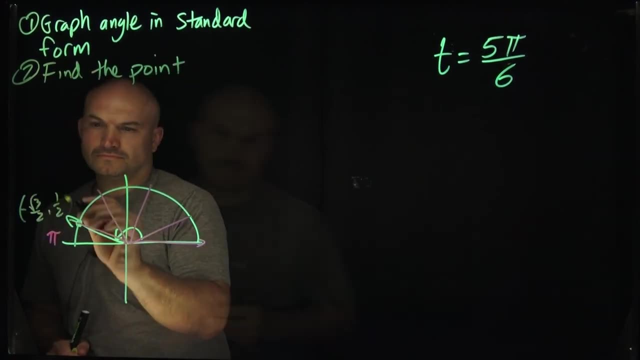 want you to be able to do is to find the corner point where your angle is going to intersect on the unit circle. Okay, and again, you can see that I found that point rather quickly and you're like: how did you know how to find that point so quickly? Well, there's one thing. 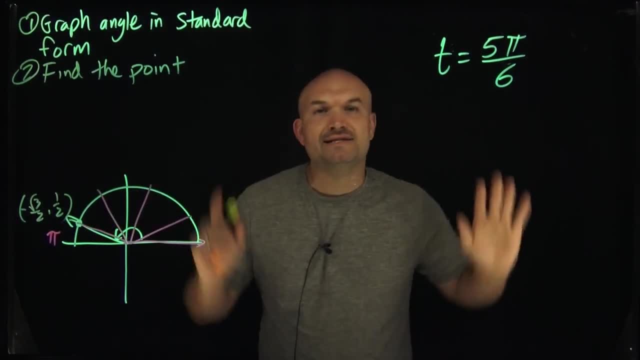 that I tell my students all the time. Like I don't want you to memorize the unit circle, Please do not memorize the unit circle because it is a complete waste of time. What I do want you to memorize is at least the: 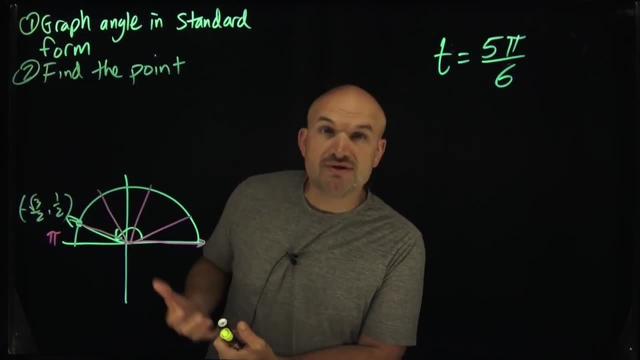 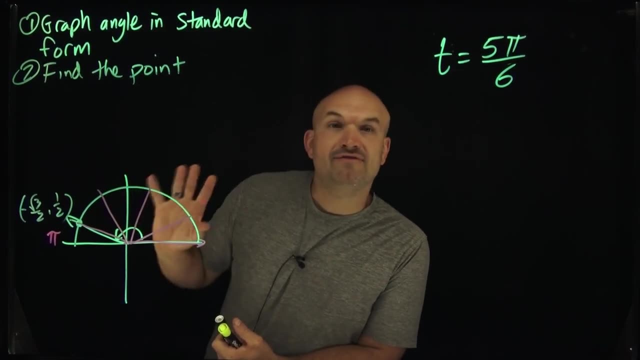 first quadrant of the unit circle, because that is something that is going to be used constantly throughout your study of trigonometry. So you do need to know those coordinates in the first quadrant. And then all I did was I knew that this quadrant, this point, right. 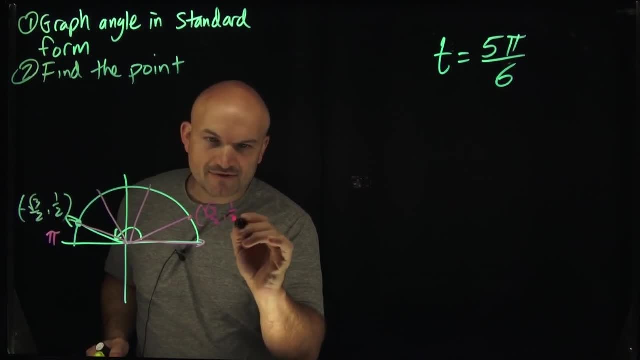 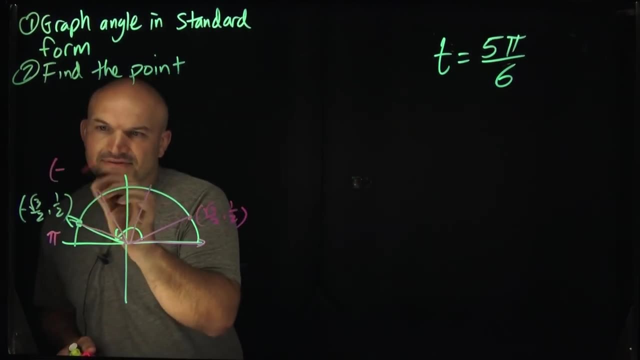 here right was kind of square root of three over two, comma one, half, all right, And that angle was pi over six. So all I did in my head was I said: hey, second quadrant, this is a negative and that's a. 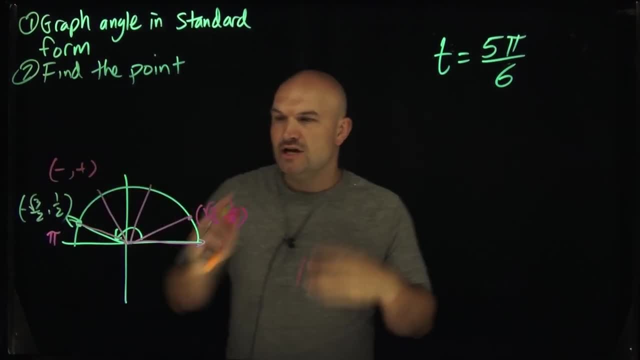 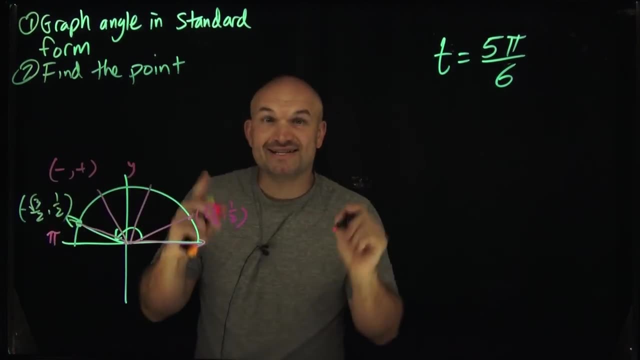 positive right. The x-coordinate is negative, the y-coordinate is positive. So all I did? I just recognized that this is a reflection about my y-axis. so therefore, the x and y-coordinates are going to be exactly the same. However, now all I simply need to do is just negate. 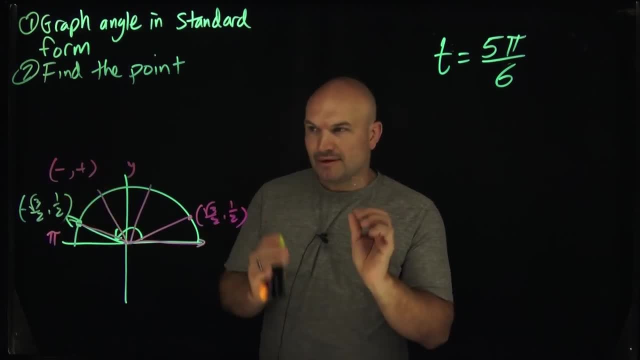 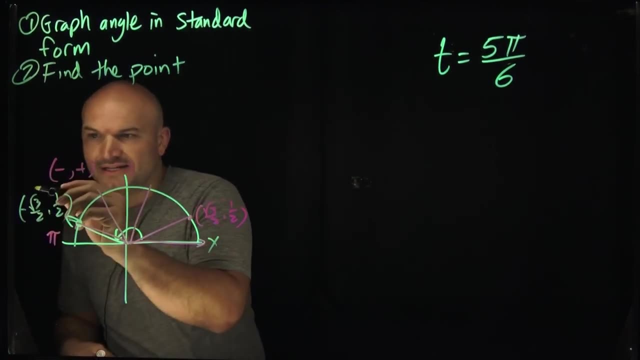 my x value. and now I have my coordinate point. okay, Now you got to remember when I graph this on standard form, this is on an x and a y-axis. So therefore, this coordinate point is going to be an x and that is going to be a y, right? 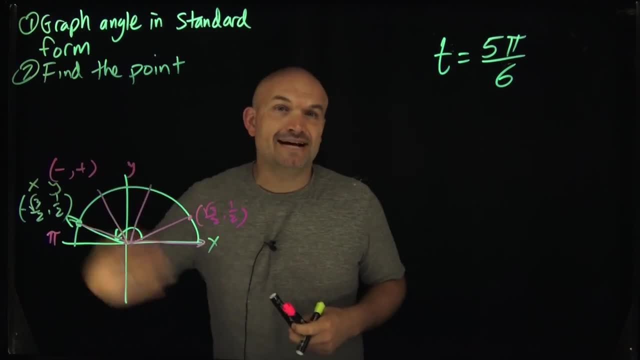 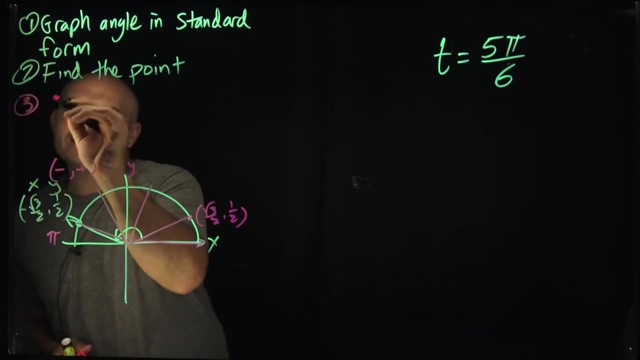 So now we have an x and a y for a given point that lies on the unit circle. That is all we need to be able to evaluate our six trigonometric functions. Why? Well, because now I can just evaluate. And again, why can you just evaluate? Well, remember, 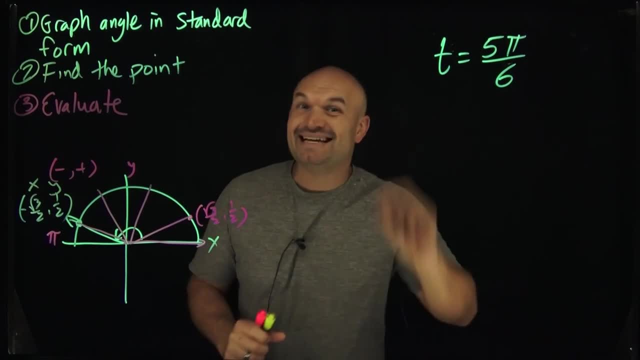 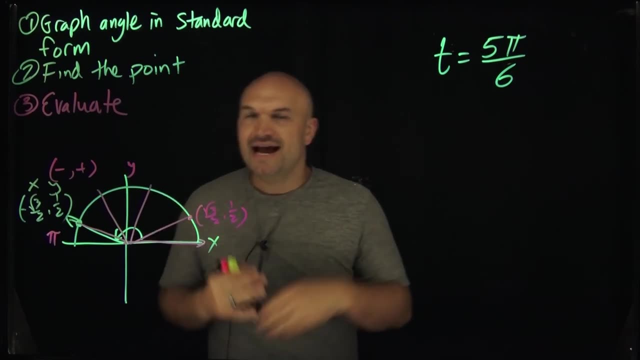 the definition of our trigonometric functions. when we have a coordinate point that is on the unit circle, sine is equal to the y-coordinate cosine's, equal to the x-coordinate tangent's. it's equal to the y over the x coordinates. 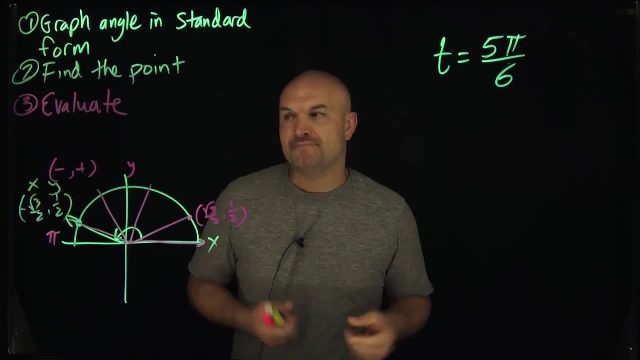 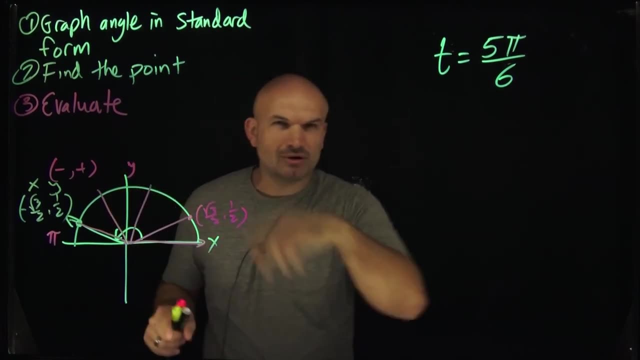 And then we have our reciprocal functions, which is just, you know, the reciprocals of that. But again, that is only for the points of our angle when they intersect the unit circle. okay, That's very important and we'll come back to that. 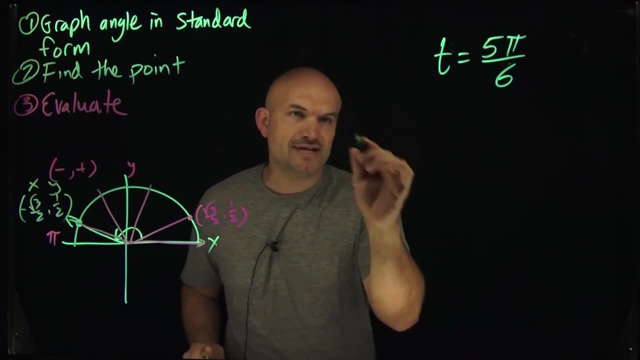 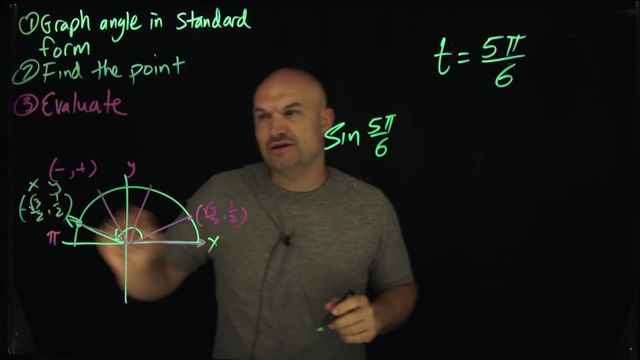 you know in some future videos. So in case you just forgot everything that I just said, if I said what is the sine of five pi over six, that is going to be the y coordinate of where that angle intersects my unit circle. 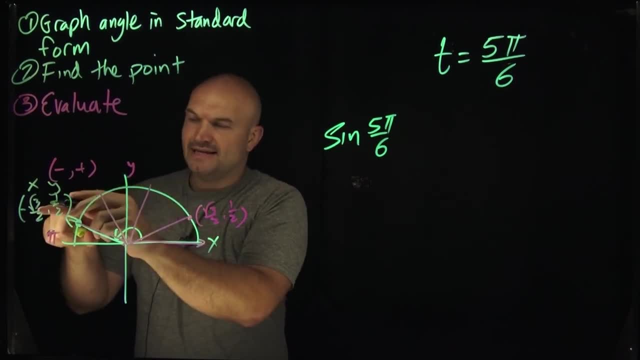 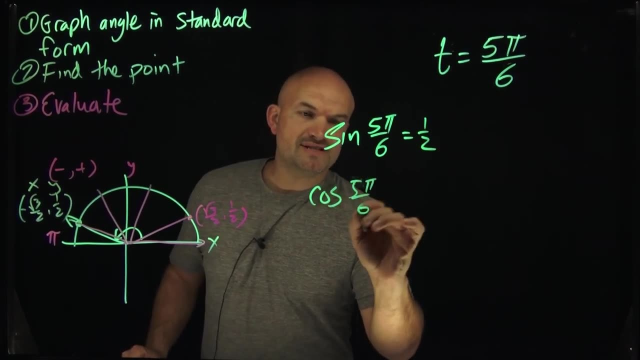 And you can see over here, right, I found the point, which in this case is negative, square root of three over two comma one half. So my y coordinate is just equal to one half. The cosine of five pi over six represents the x coordinate. 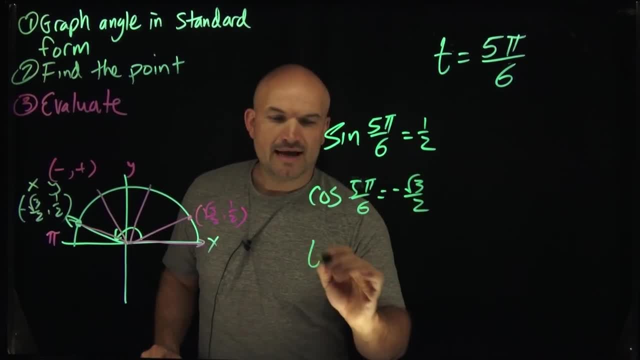 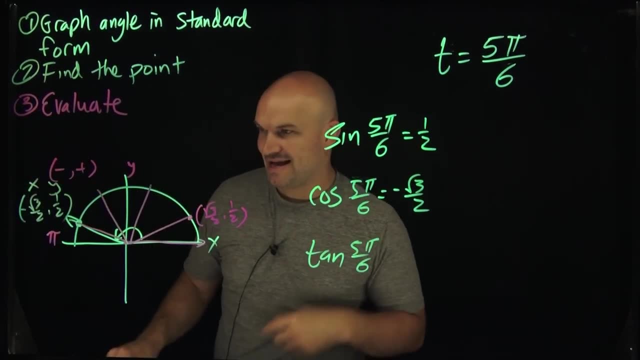 which in this case is gonna be negative square root of three over two, And then my tangent of five pi over six is going to be the y coordinate over the x coordinate. Now, here we're gonna have a little bit of math, but that's okay, let's have a little fun. 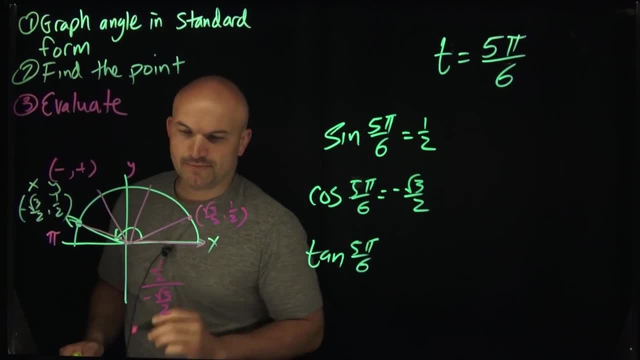 So I have a one half divided by a negative square root of three over two. Okay, now, hopefully you recognize that I have a fraction of my numerator, fraction of my denominator. Well, guys, both those fractions are being divided by two. So what I can do is I can just actually simplify this. 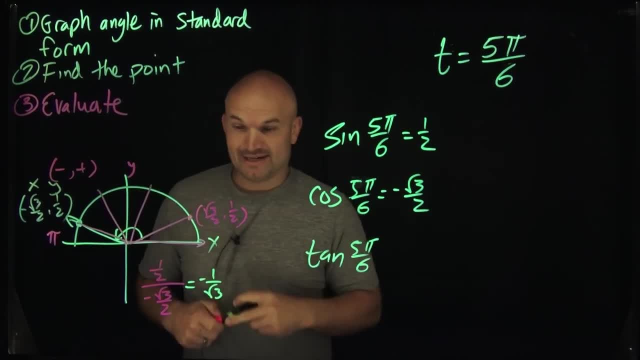 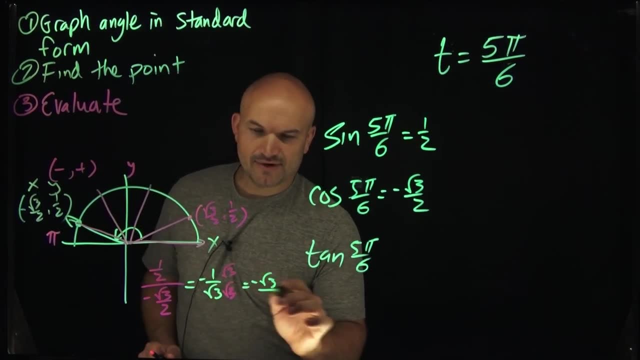 to a negative one over a square root of three. Now if I wanted to simplify that, I could just rationalize the denominator by multiplying by a square root of three on the top and bottom, and I'll get a negative square root of three over three. 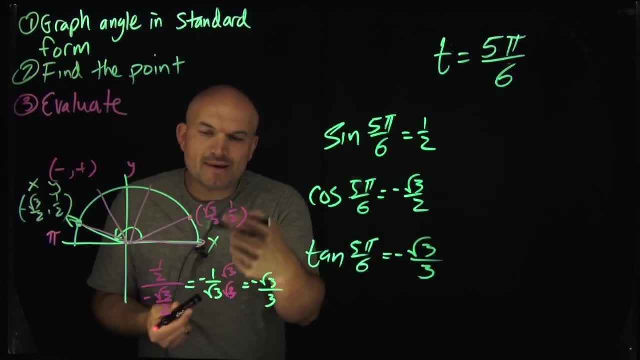 Okay, and if you didn't like that idea of how I just got rid of those twos, multiply a two on the top and the bottom right. That will get rid of those twos very quickly from there. All right, so now it's time to do our reciprocals. 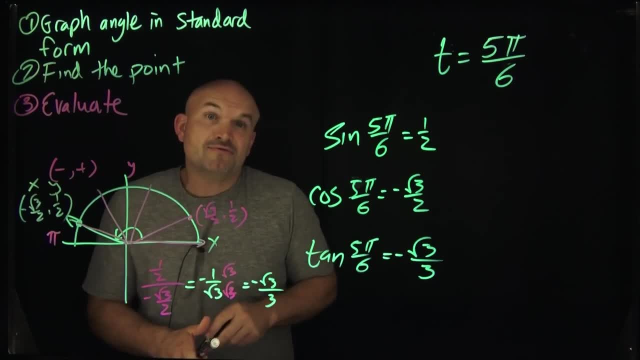 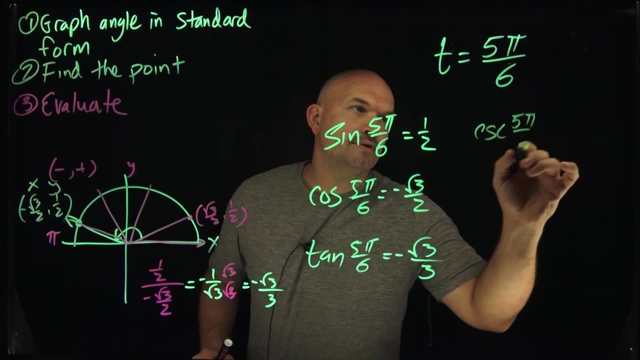 and hopefully we don't have to do as much math over here because we can just flip over answers that we have over here. So let's go ahead and figure out what we got. The cosecant of five pi over six is just gonna be one over y. 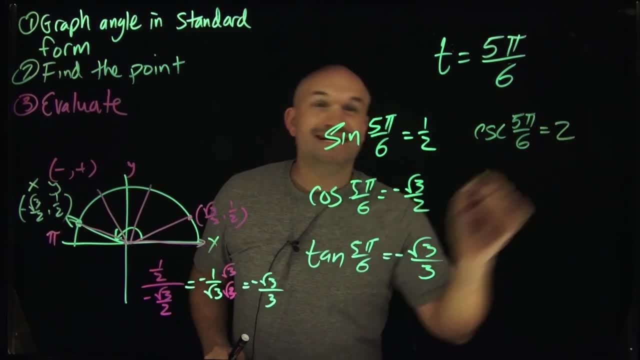 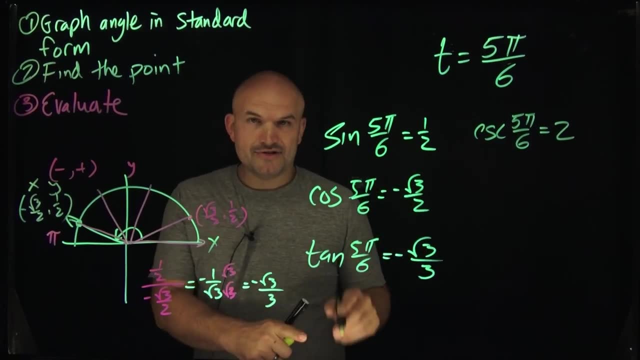 which again one over y, was just going to be the reciprocal. so that's gonna be pretty easy. That's just gonna be a two. The secant of five pi over six is going to be one over x In this case. that's gonna look a little weird. 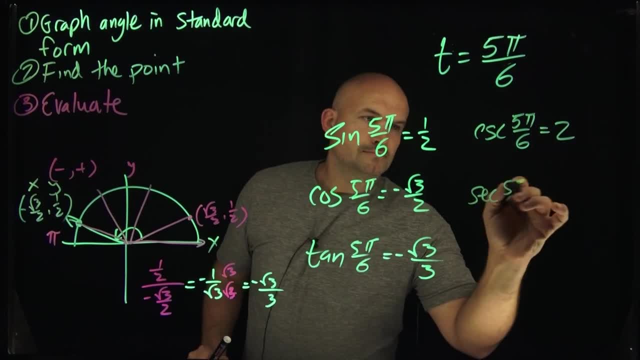 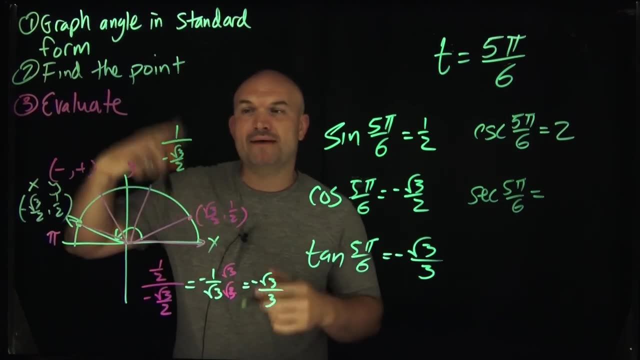 so I'm actually gonna do the work over here, All right. so in this case we're gonna have a one over a negative square root of three over two. Again, what I'm gonna do is multiply by my reciprocal, on the top as well as on the bottom.